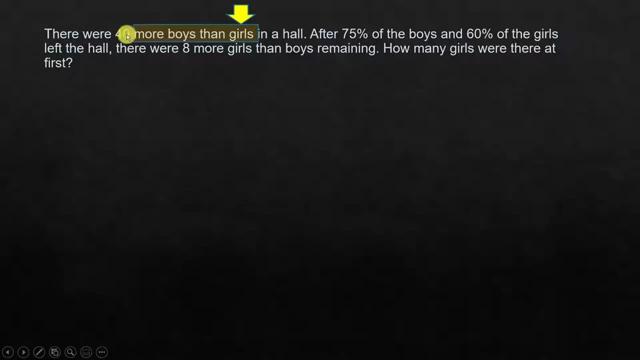 So let's draw a model for this statement. There were 40 more boys than girls, So draw a model for girls. This is the box that we have drawn for girls to represent the number of girls, And for boys it is the same quantity plus 40.. 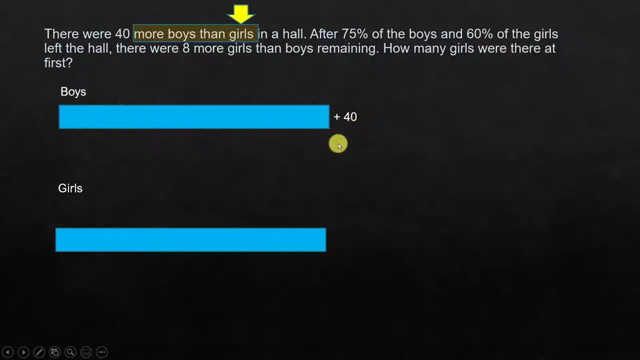 So that is the number of girls. So that is the number of boys that we have. Now you can see that there are two parts here. When we are representing the boys, we have an unknown quantity here. We don't know the value of this quantity. 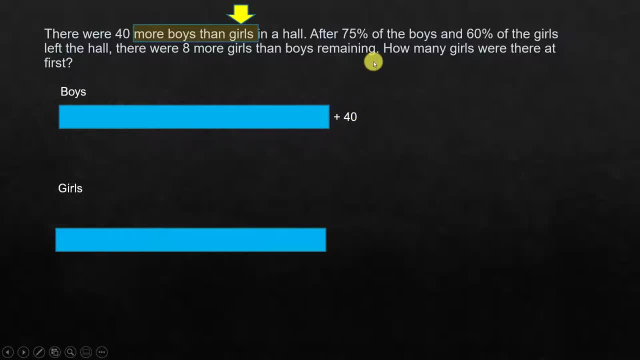 Plus 40, that is a known quantity After 75% of the boys and 60% of the girls left the hall. So what happens then? Let's try to put this down: 75%. We will represent 75% of the girls. 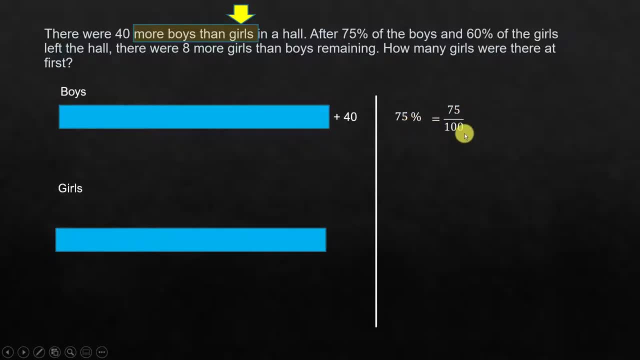 75% in terms of fractions, can be represented as 75 over 100, which, on simplification, gives 3 over 4.. Similarly, now, when we say 3 over 4, what it means is the total of this when we divide this into 4 parts. out of the 4 parts, 3 parts left. 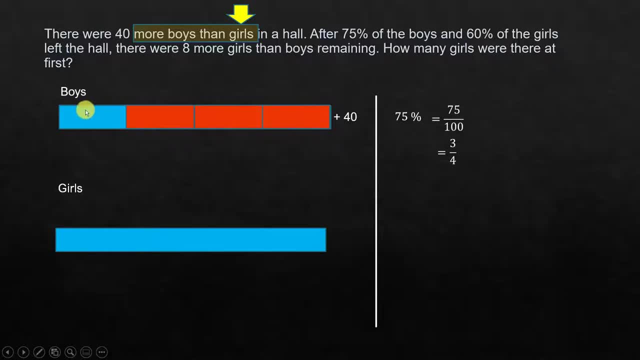 Because 75% of the boys left. This is for the unknown quantity Right, Right, And now we also have a known quantity. So that is 3 fourths of 40. That is the number of boys who left. So that is equal to 30.. 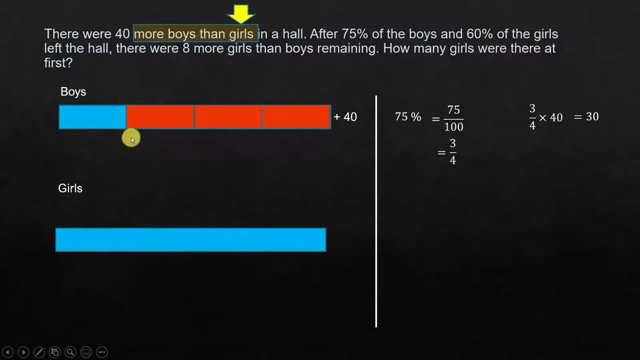 So there are two things here Of the unknown component. if we divide the unknown component into 4 parts, 3 of the parts represent the students that left the hall And from this known quantity, 40, 30 students left the hall. 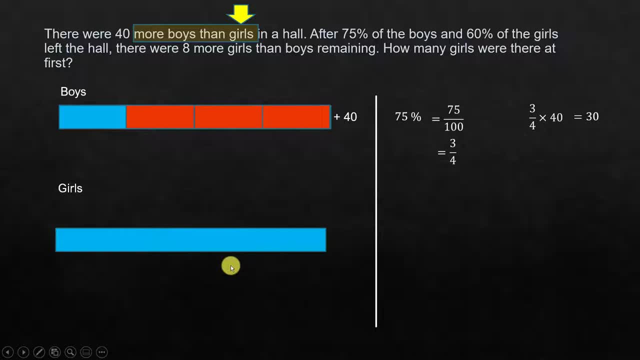 The remaining is 10.. Now for the girls, it is 60%, And 60% can be represented as 60 over 100. Or, on simplification, it becomes 3 over 5.. Again, here it means we are going to divide this total into 5 parts, out of which 3 parts leave the class, which leaves us with 2 parts. 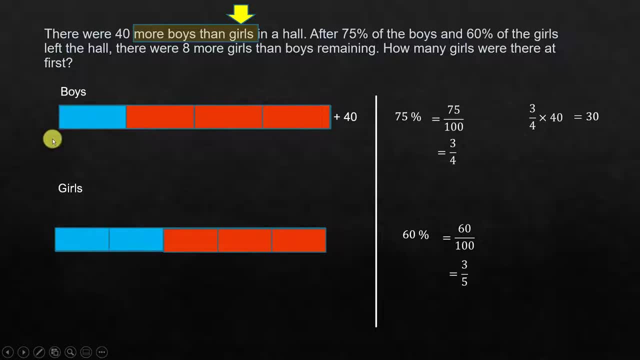 Now you can see that for the boys and the girls, the unknown quantity, the total unknown quantity, the size is the same, But this small here, the unit size of this went here is not the same as the unit size of this. 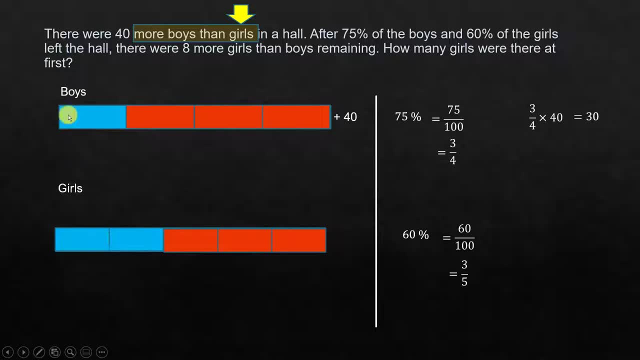 How do we know? Because the same quantity here has been divided into 4 equal parts, whereas here the same quantity has been divided into 5 equal parts. So obviously this unit is going to be smaller than this unit, But we don't know how much smaller, and so on. 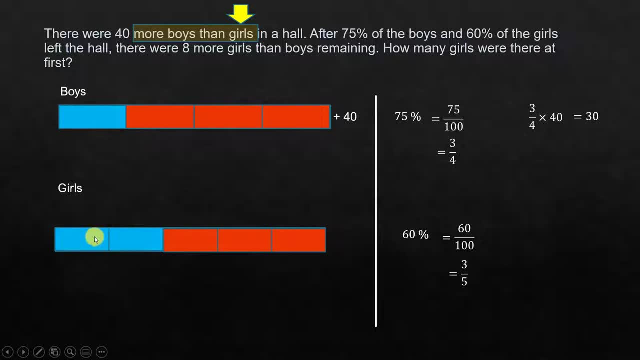 So we don't know the relationship between the two units, But we established that relationship. We can take this as a whole and this as a whole and then see how we can try to come with a unit size of the same units of the same size. 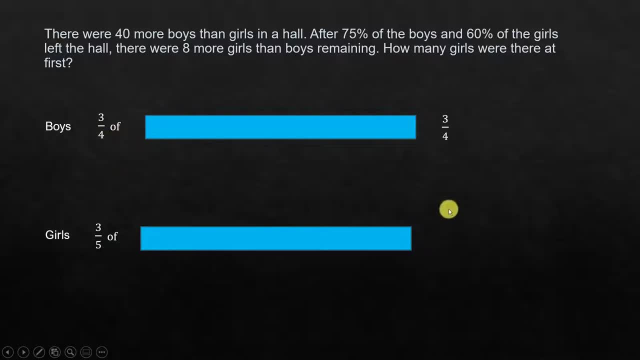 Let's go back: 3 by 4 of the boys and 3 by 5 of the girls. right, We have two values: 3 by 4,, 3 by 5, and both. this is 3 fourth of this unit and this unit. 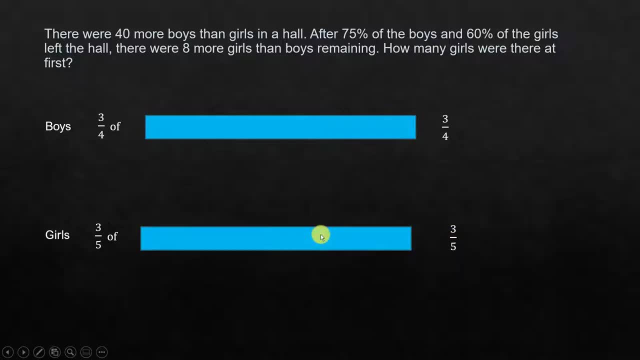 size is the same as this unit. Here is 3 fifths of this unit. Now, what we are going to do is find the LCM of 4 and 5, which are the denominator, because we want to end up splitting this into smaller units of the same size. 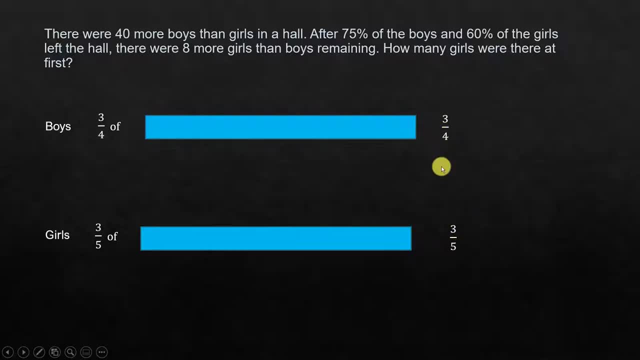 So here, 4 and 5, the LCM is 20.. So 4 times 5 gives 20.. Similarly, here, 5 times 4 gives us 20.. And when you Multiplication, When you multiply the denominator with a value, you have to multiply the numerator with the. 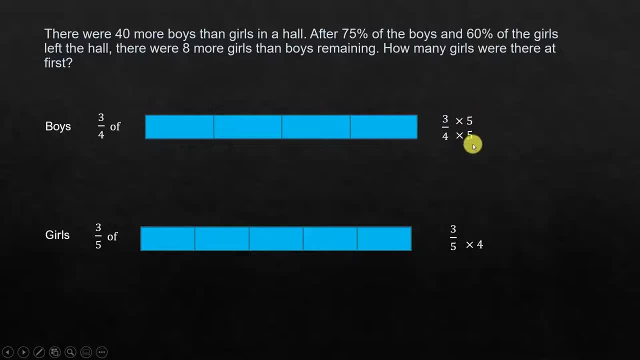 same value, So that 5 over 5 is actually 1,, which means the value of this does not change, Again the same. here we multiply the numerator with 4, so that 4 over 4 is 1, and the value: 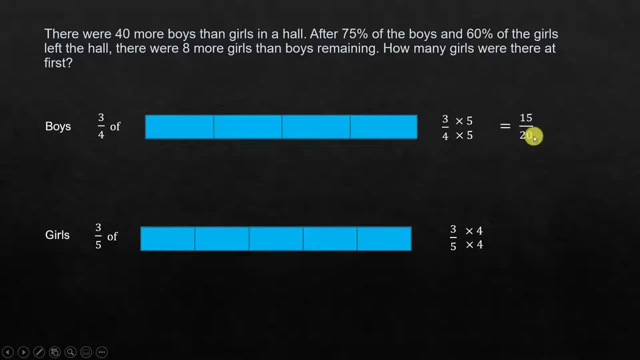 does not change. So this becomes 15 over 20, and here it becomes 12 over 20.. What it means here is see, we had 4 parts in the beginning. Each of these 4 parts, we are going to divide it into 5 smaller units of the same size. 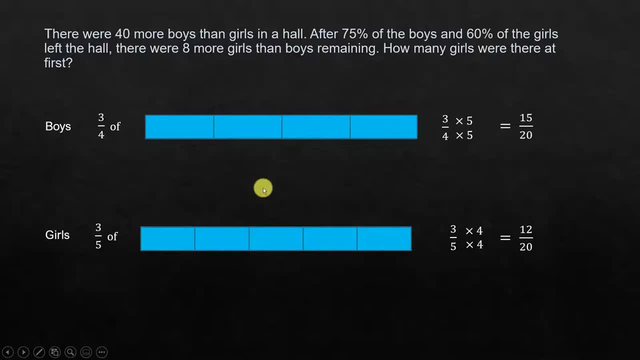 so that in total we end up with 20 units. So you can see here we are going to divide this into 1, 2, 3, 4, 5 smaller sized units. Here we had 5 units and each of this unit is going to be divided into 4 smaller units. 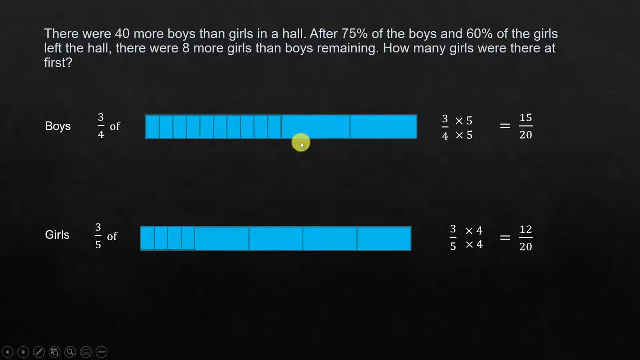 Right, When we continue doing that, 5, 5, 5.. We are doing it again: 5, 5, 5.. 5, 5, 5.. We are doing it 4 times, so that's 20 units here. 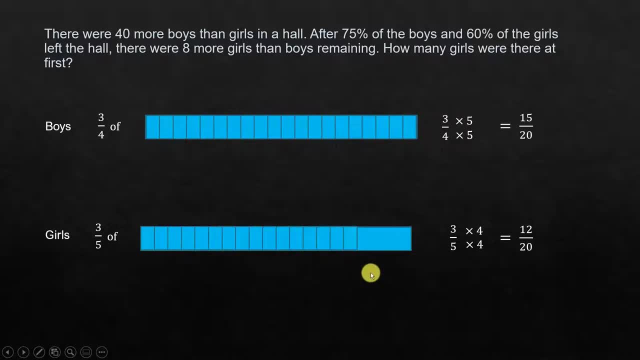 Here: 4, 4,, 4,, 4, and 4.. So 5 times that gives us 20 units as well. So this is how we, once we do this now, we are able to compare them easily. 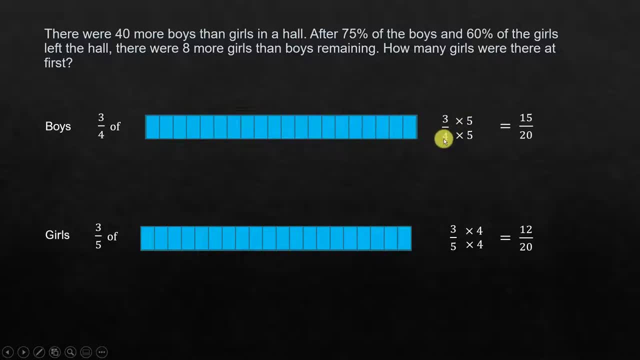 And out of this, this is 75%, which is the number of students who left right Out of 15, out of 20 left. So 15 units left Left, with 5 remaining units. Similarly, here, 12 units have left. 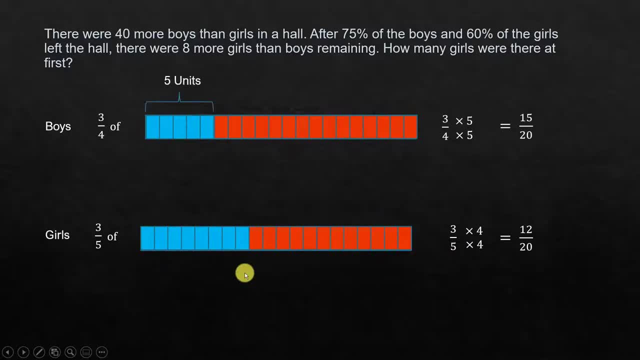 So we will be left with remaining 8 units here. So now we go back and apply this. So, for the unknown quantity, we know that we are left with 5 units for the boys and 8 units for the girls. So you can see here, boys, what is left is 5 units plus 10 plus 30.. 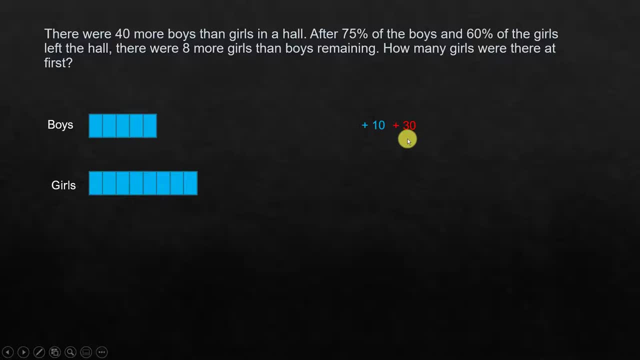 We know that this 30 is the number of students who left. We know that this 30 is the number of students who left, The number of students who left for the known quantity, So we'll remove that Now. for boys, what is left is 2,, 3, 5 units plus 10.. 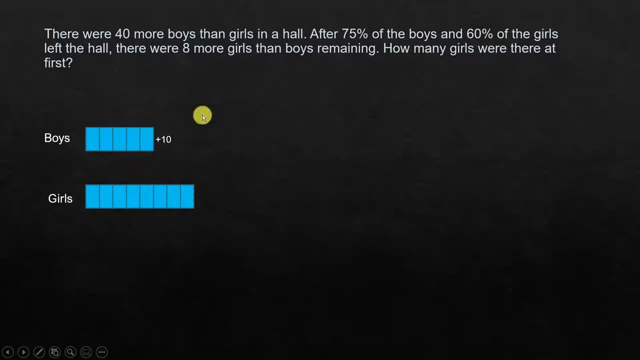 And girls. it's 8 units And it says after the 75% of the boys and 60% of the girls left the hall, there were still 8 more girls than boys remaining, which means the number of girls is more than the. 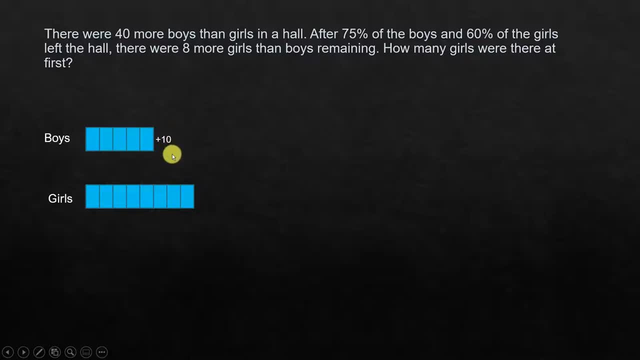 number of boys, And that is After, after this 10. so to represent this 10, let's put this in a box, right? and if I just put a slightly bigger box, to differentiate with this from the rest of the units, because the sizes may not be the same, but we don't know yet. so the 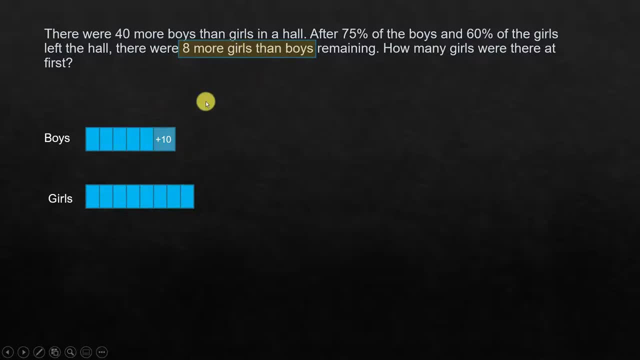 girls is how much more? eight more girls than boys. and that is from here to here. so that is eight and from here, if you draw a line, you can see that from here up to here, these three units, that is going to be equal to 10 plus 8, right? so 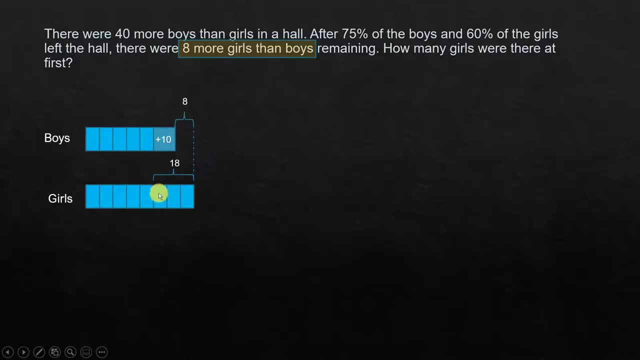 that is going to be 18, so three of these units is equal to 18. one unit is 18 divided by 3, so one unit is 6. now we have found out that one unit is six, and earlier we have also realized that girls had a total of 20 units, right? so if we forget about the number of 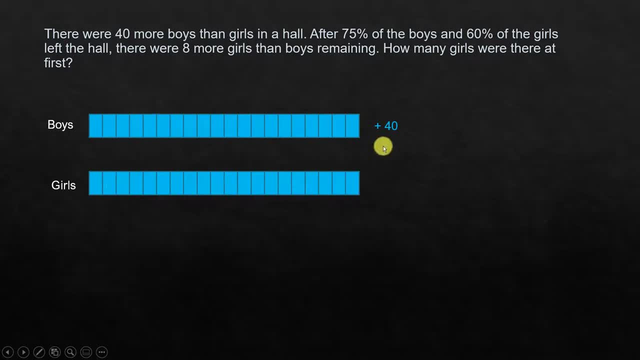 students who left originally. boys had 20 units plus 40. girls were 20 units and we know that each unit is 6, so number of girls is 6 times 20, which is 120 you, so the number of girls present at first is equal to 120. hope this was helpful. we 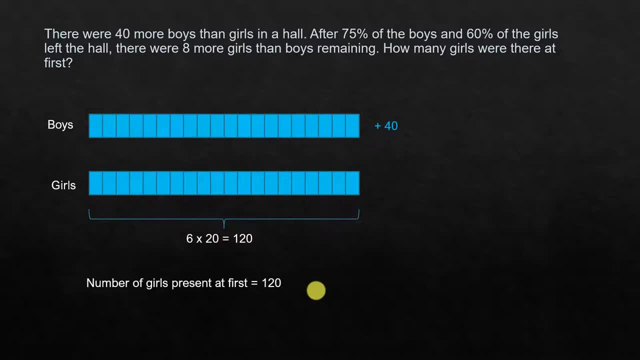 went through a slightly longer route to understand how we do the LCM and all that stuff. but in general, if you don't want to go through that route, let's just summarize what we did. if this is a problem, we again go by the same thing: more boys than girls. so girls is our reference quantity. so we draw a model. 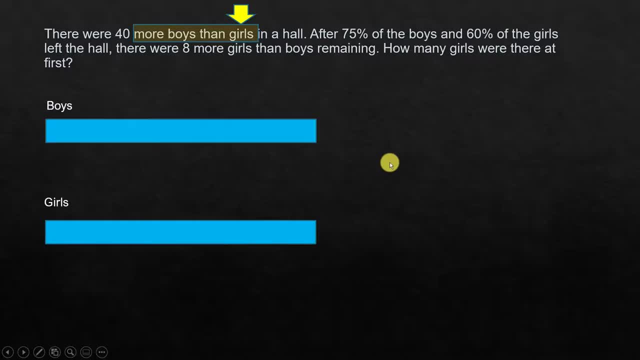 for girls, and then we draw a model for boys and it talks about 75 percent of the boys. we know 75 percent means 3 by 4 or plus 40 as well here, and so we are going to divide this into four parts here. we are going to divide them into five parts and to make the unit sizes the same. what we are. 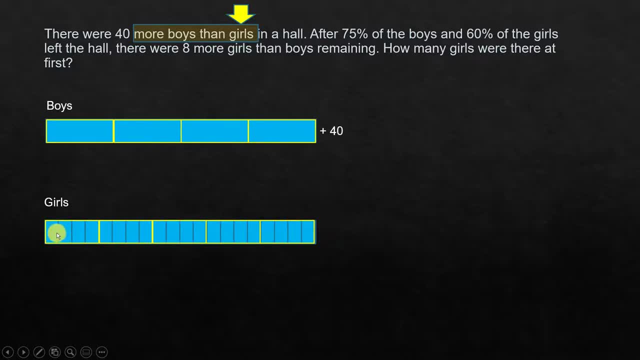 going to do here is divide these into four each, so total 20 units. divide this into five each resulting in 20 units. and now we are going to separately find out 75 percent, or three by fourth, of that would be this much left right. so how many units? minus 15 units here and minus 30 of the known? 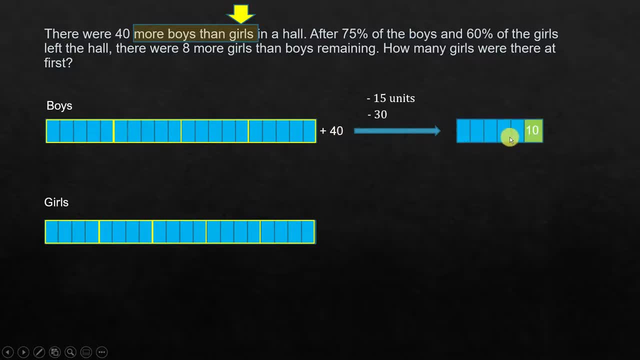 quantity. that will leave us with one, two, three, five, and we are going to divide this into four parts and to make the unit sizes the same units- and the known quantity is 10 for the girls we know- 60 percent would mean 12 units will have to. 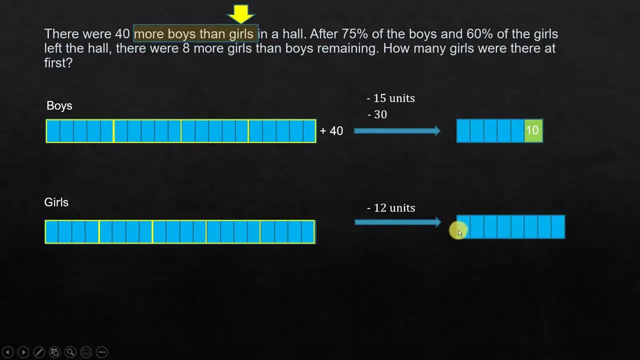 be removed or they left. so we are left with eight units here and after this, for the kids who are left, there are eight more girls than boys, which means up to here is eight right, there's a gap here. so total is 10 plus 8.. 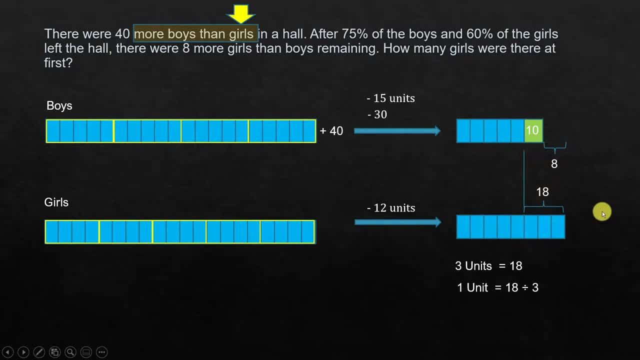 it is 18, so three units is 18. one unit is 18 divided by 3, which is 6. so the total number of girls is 20 units. that is 20 times 6, which gives us 120.. so this is how we solve the problem. 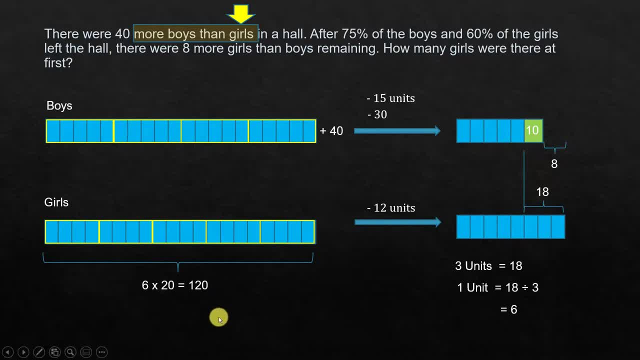 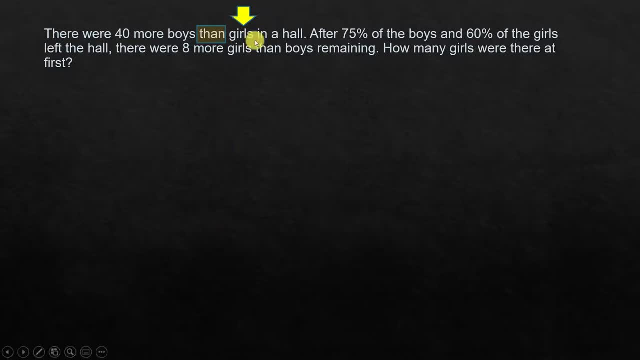 i hope this was helpful. next we move on to see how we can solve the same problem using algebra. there were 40 more boys than girls. the same logic applies here: girls is our reference to girls and reference. so we will take the number of girls in the hall to be x and the number of boys is 40 more. 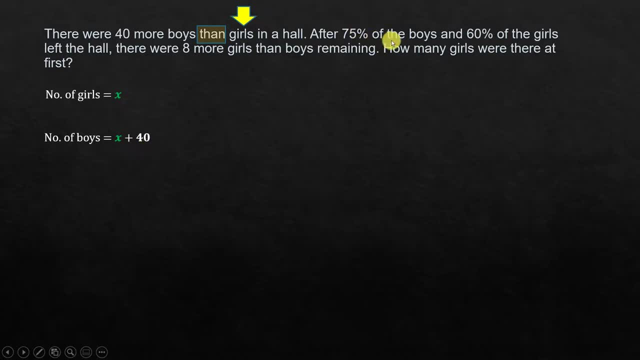 so x plus 40. and after 75 percent of the boys left, so minus oh, sorry uh. and 60 of the girls left the hall. so for the girls minus 60 percent, which means remaining is 40 percent of x, for the boys 75. 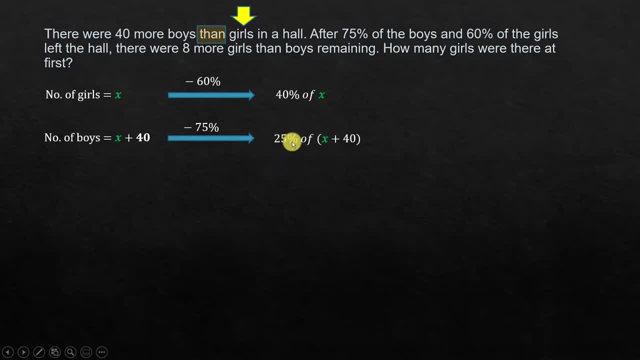 left, so it's going to be 25% remaining of x plus 40. Now at the end, we know that there are eight more girls than boys. Let's write down girls and boys. So there are eight. right now there are eight more girls. 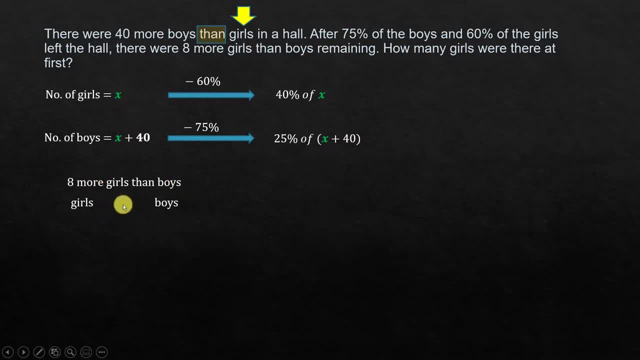 than boys If we were to make them equal, girls and boys, because we need an equation here. so to make them equal, what we need to do is add 8 to the boys section, so that the number of girls and the number of boys would be equal. so 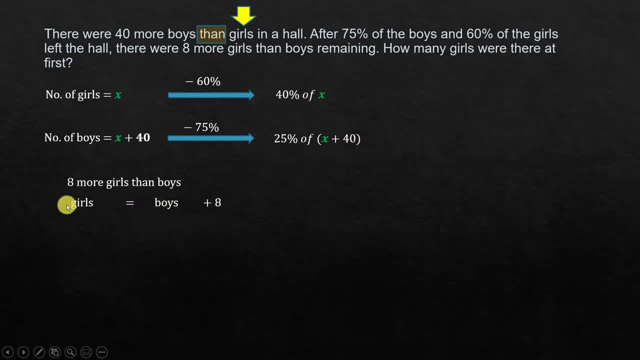 that we can come to create an equation here. So number of girls is 40% of x and here boys is 25% of x plus 40, and to make them equal we have to add this plus 8 as well, On simplification. 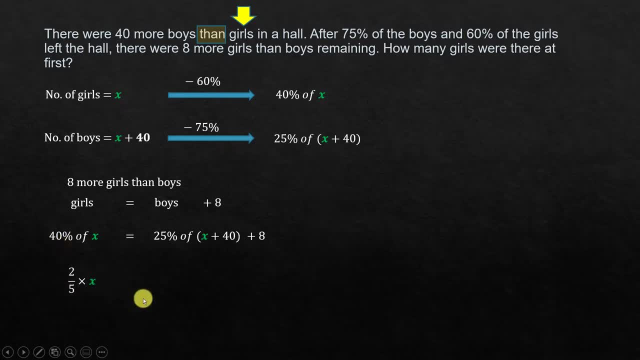 this would become 2 by 5 of x, and that is equal to 1 by 4 of x plus 1 by 4 of 40, 1 by 4 of x plus 1 by 4 of 40, which is 10 plus 8.. 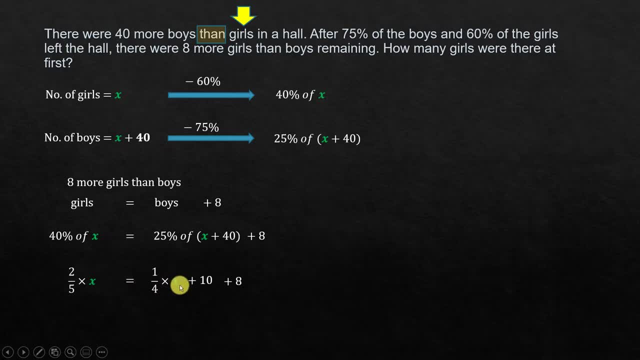 Alright, so now we want to remove. bring all the x terms to one side, so that would become 2 by 5 of x, minus 1 by 4 of 40.. by 4 of x, which is equal to 10, plus 8, which is 18.. 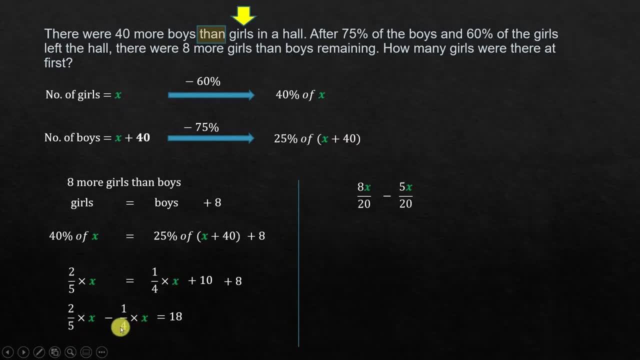 Now this, here again the same. we are going to find the LCM of 5 and 4. so here you are going to multiply times 4 times 4. 4 times 2: here becomes 8, 8x over 20 and here it is times 5 below to make: 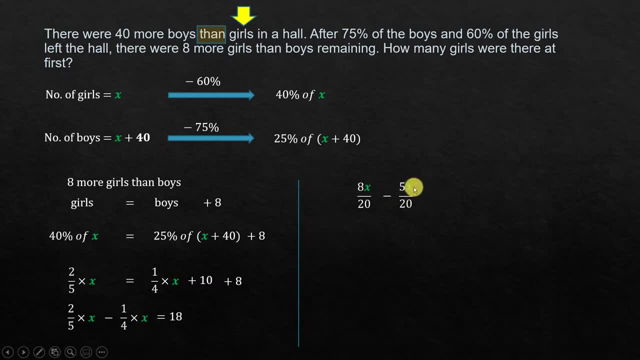 it 20 and on top times 5, so that becomes minus 5x over 20, which is equal to 18. that is 3x. so 8x minus 5x over 20 equals 18, so that is 3x is equal to 18 times 20, x is equal to. 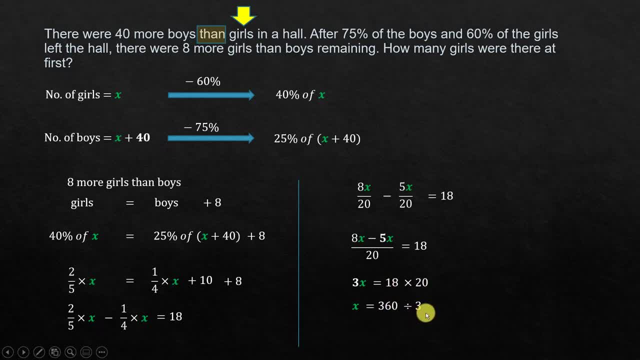 18 times 20 is 360 divided by 3, so x is equal to 120.. So the number of girls present at first, which is equal to, if you see here, number of girls, is x actually, so the value is 120.. So this is how we solve. 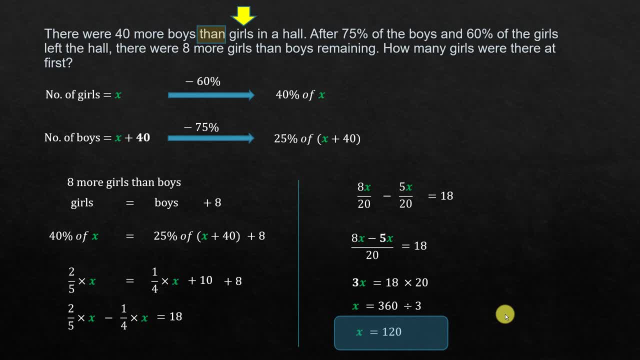 this problem in algebra. So hope this was helpful. If you have any questions, doubts, please post your questions- comments- in the comment section. Do not forget to subscribe and like the video, share it with your friends. Have a great day and if you have any more questions, 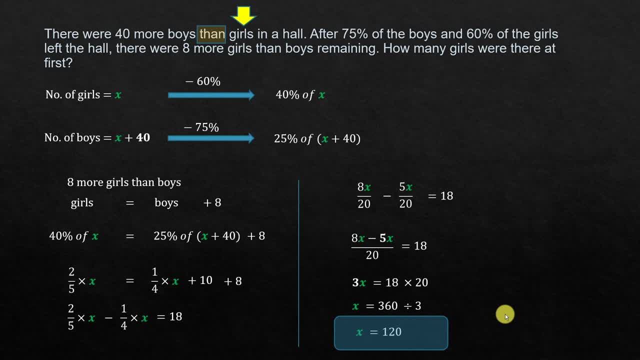 that you would like me to solve. please let me know. I will try to get you as many as possible. Have a great day. Thank you and bye.